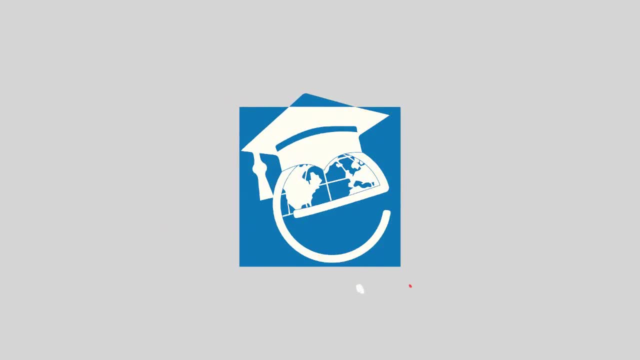 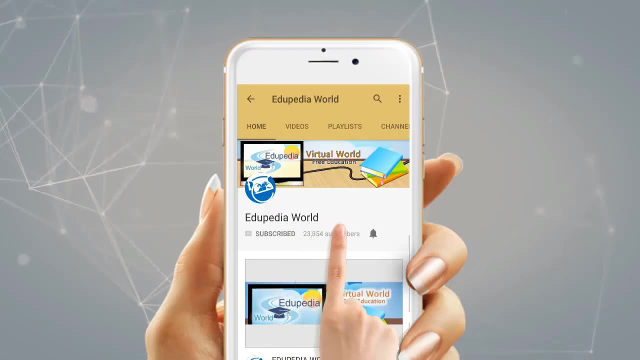 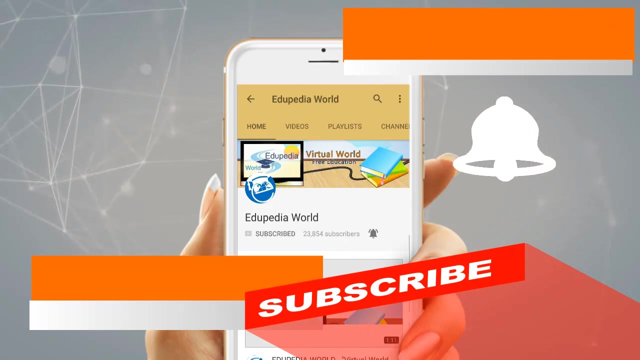 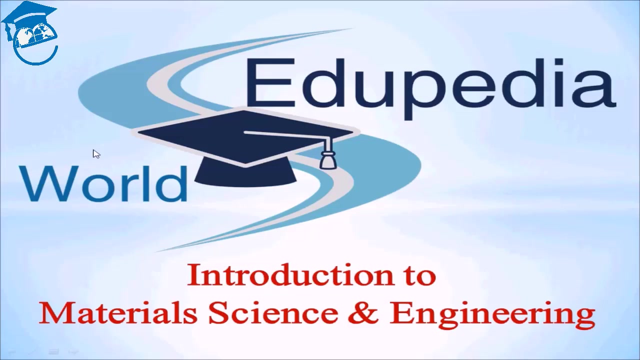 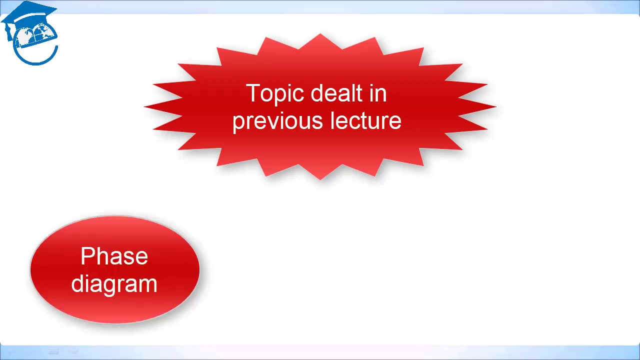 Hi everyone. welcome back to the course on Introduction to Material Science and Engineering offered by Edupedia World. In the previous set of lectures we discussed about phase diagram and we saw the different kind of invariant reactions that takes place. In addition, we saw the iron carbon phase. 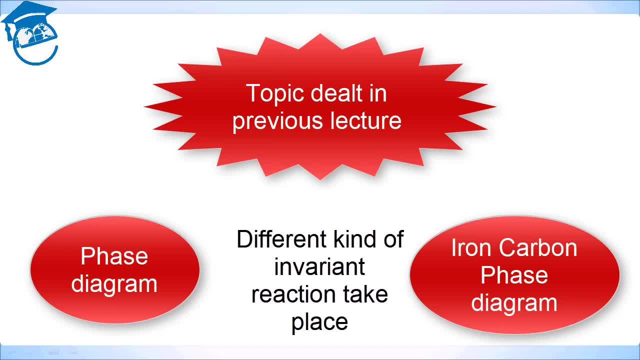 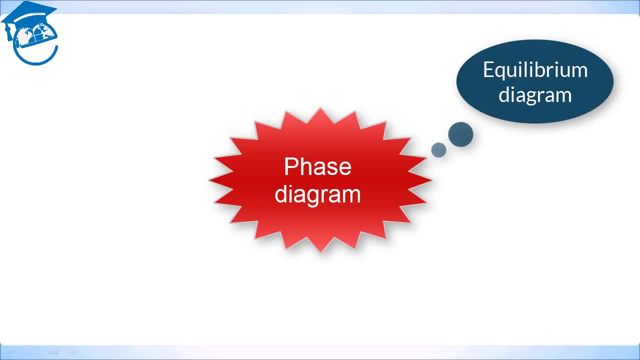 diagram. One thing which I mentioned while discussing phase diagram is that phase diagram is a equilibrium diagram. It does not take into account the rate of a reaction or the rate of phase change, But in reality, any phase transformation has a rate of reaction. 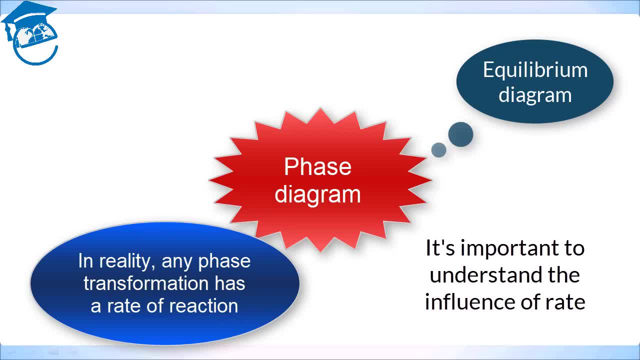 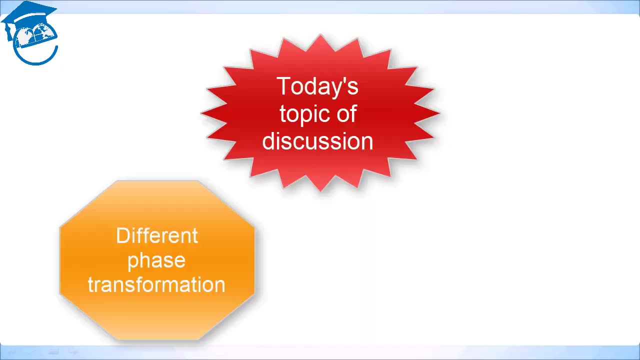 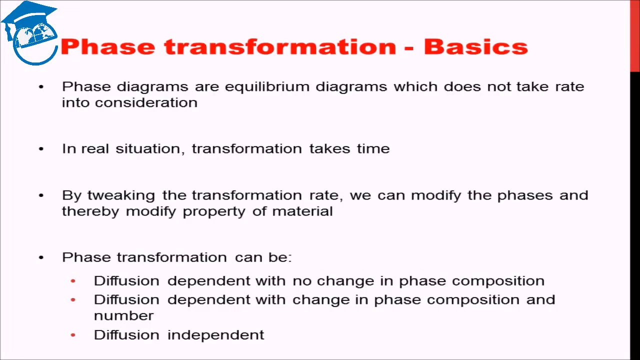 Therefore, it is of pivotal importance to understand what will be the influence of rate on different phase transformation. That is what we will study in this chapter. We will discuss about different phase transformations and how is the kinetics of different kind of phase transformation. So let us begin with the basics of phase transformation. As I mentioned, the phase diagrams are equilibrium. 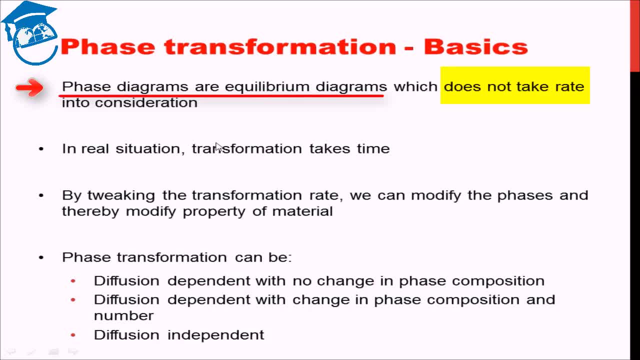 diagrams that does not take rate into account, right, Because they are equilibrium diagram by definition And in real scenario, obviously, transformation takes time. Therefore, this fact that transformation takes time can actually be an advantage to us. We can tweak the transformation rate by: 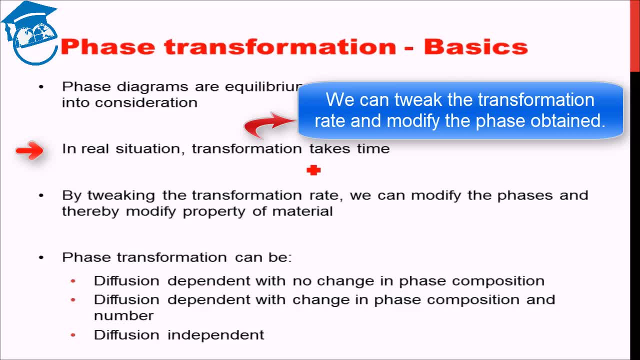 different processes and thereby we can modify the phase that we can obtain, because phase diagram gives you a specific phase that can be obtained But in reality, since the rate can be different under different circumstances, we can change the rate of reaction or the change the rate of heat treatment, and thereby we can modify the phases that can. 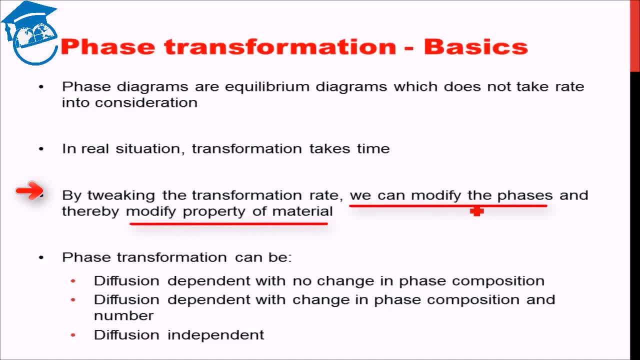 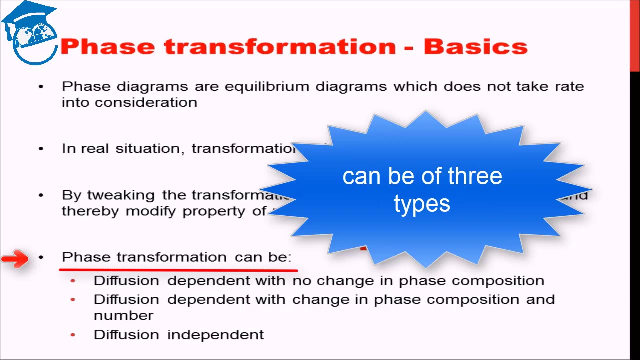 be obtained, And this change in the phase that can be obtained will lead to a change in the ultimate property of the material, Because the property of a material is determined by the type of phases, the properties of phases right. The phase transformation can be of three kind. It can, broadly speaking, either be diffusion, 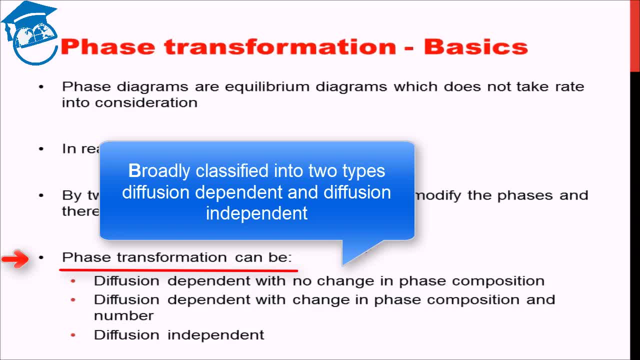 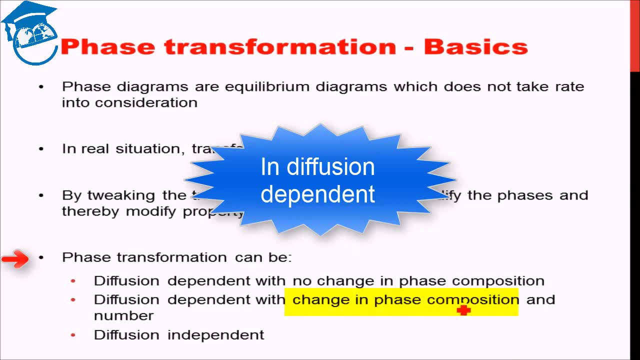 dependent or diffusion independent process. in the diffusion dependent process there can be either a change in the composition of the phase or there can be no change in composition of phase. An example of diffusion dependent process with change in composition of phase is the Basically eutectic reaction- Eutectic or eutectoid reaction, Whereas diffusion independent process we will see one of the most important example that will be widely used. that is widely used in the case of iron and steel is martensitic transformation. 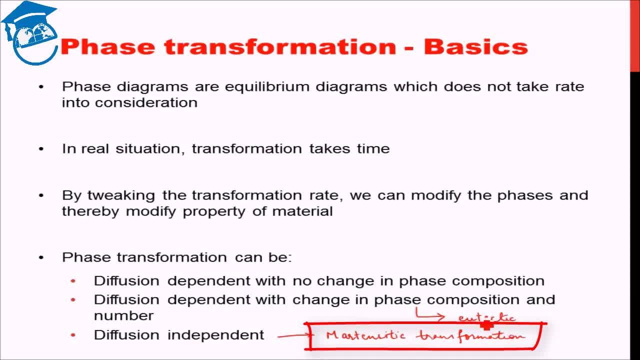 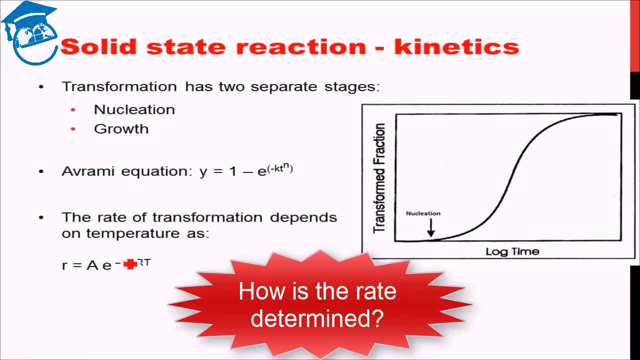 Okay, Now how is the rate determined, or what are the factors that affect the rate of the reaction Transformation phase? transformation consists of two different stages. The first stage is nucleation and the second is growth. What is nucleation? What is nucleation? Nucleation is basically generation of the nucleation. 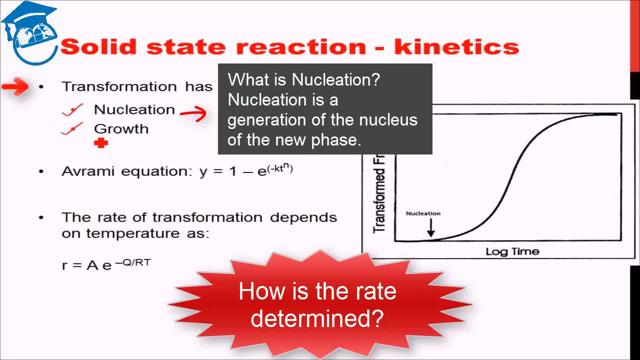 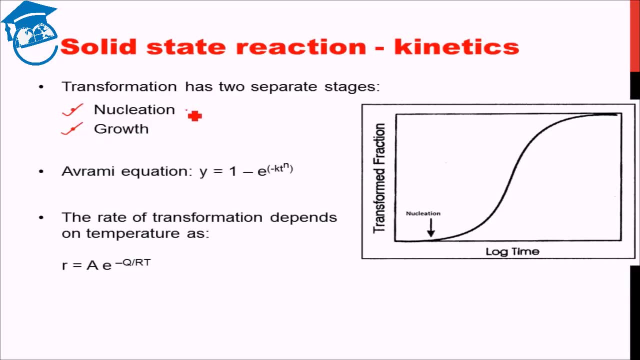 Of the new phase. Only once the new nucleus has generated can the growth begin. So nucleation can take some amount of time on its own And once the nucleation has taken place, once you have a nucleus, then that nucleus starts to grow. The growth also has a particular kinetics behind it. It follows certain kinetics, which is dictated by diffusion. 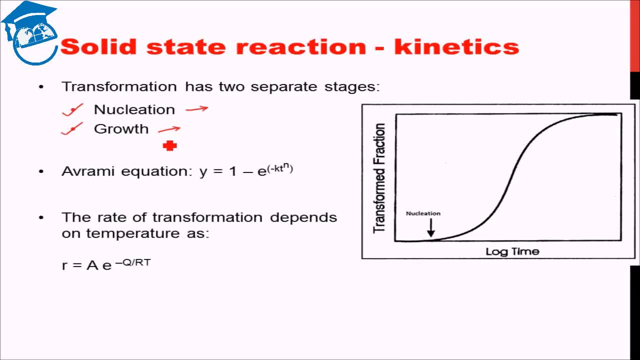 Okay, So the nucleation rate depends on what is the driving force. Suppose you are trying to freeze water, The nucleation rate will be faster. lower the temperature: If you keep the temperature at zero degrees Celsius, then the rate of nucleation will be quite low. On the other hand, if you take the water suddenly to minus 20 degrees Celsius, the rate of nucleation will be lower. 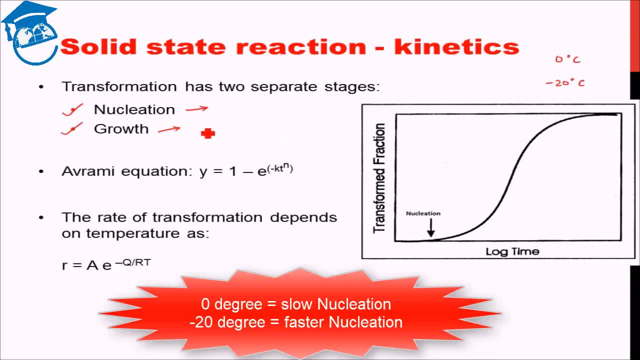 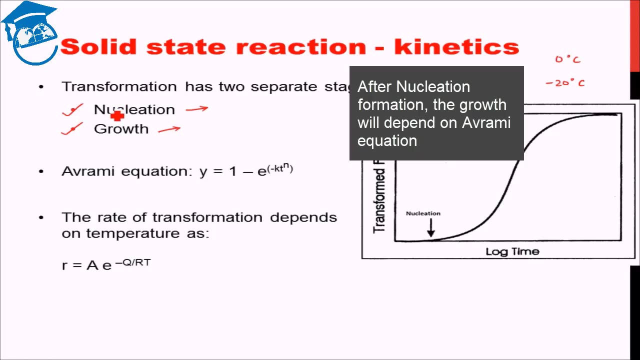 Okay, So the nucleation rate will be very, very fast. Thereby, nucleation will not take much time. Therefore, what is the? how much is the driving force for the transformation to take place That will decide the rate of nucleation? Once the nucleus has formed, the growth will depend on what is known as Abrami equation. Okay, 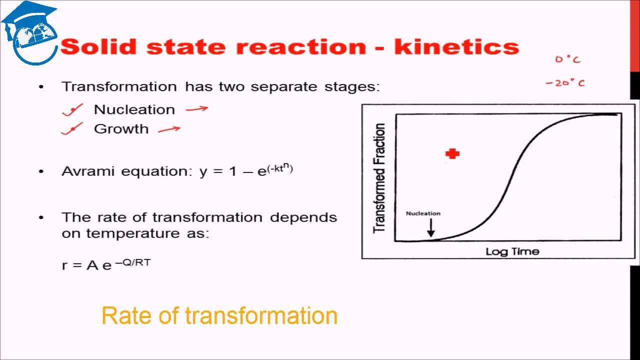 The rate of transformation will follow this trend. This is the graph which shows on the x axis time in the logarithmic scale, and the y axis is fraction of transformation that has taken place: Zero to one. Initially, nucleation will take a certain amount of time, which will depend on the driving force. Once nucleus has taken place, it will. the transformation will follow this trend. 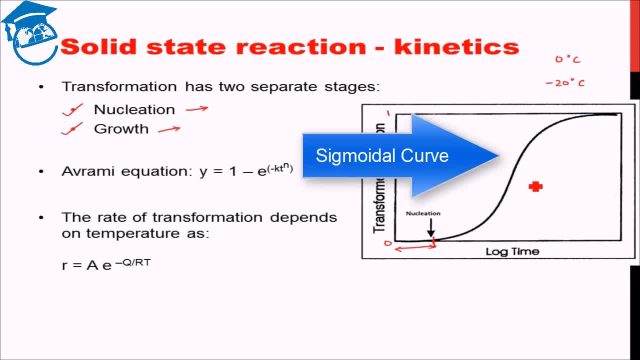 The rate of nucleation will follow a sigmoidal curve. The rate of transformation, the fraction of transformation. Initially, the transformation picks up, It becomes very fast and ultimately it again slows down. This relation is represented. this kind of graph is represented by this relation: Abrami equation. Fine, Now suppose that the driving force was very, very low. Then what would have happened? This nucleation will take a certain amount of time, So the rate of nucleation will take a certain amount of time. Once nucleus has formed, the growth will depend on what is known as Abrami equation. Okay, 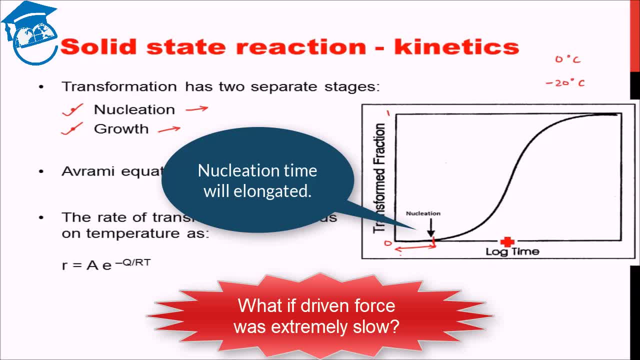 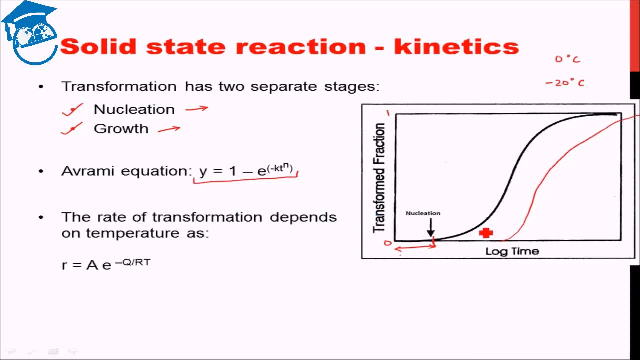 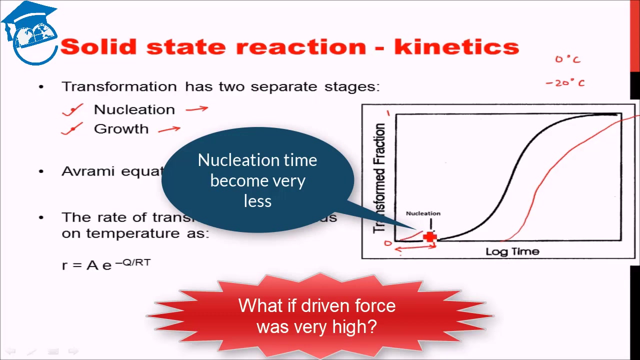 The nucleation would have elongated the time for nucleation and basically we would have had a graph like this Right, So more time would have effectively taken. If the nucleation happens instantly, then there will be no time required for nucleation or very less time required for nucleation. Thereby the transformation starts immediately, and the fraction conversion against time would have been something like this: 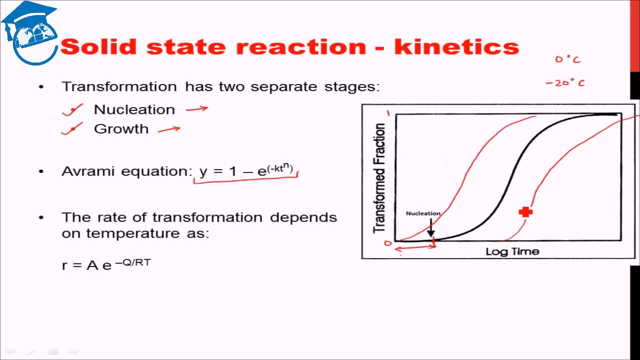 Like this: Fine Now. the rate of transformation also depends on the temperature. So this rate of transformation, how fast it is transforming, will depend on temperature, by this equation, Since it is a diffusion driven process. If it is a diffusion driven process, higher the temperature, higher will be the rate of diffusion. Higher the temperature, higher the rate of diffusion. 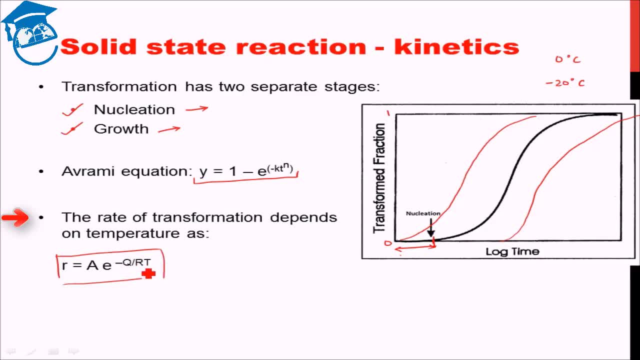 Lower this Effectively. this is less negative. This is high. Thereby, rate of diffusion is high. So increasing temperature leads to rise in the rate of transformation. This is mainly because of diffusion being dependent on temperature. So if the temperature is increased in, let's say, this case and let's assume that nucleation is not affected, 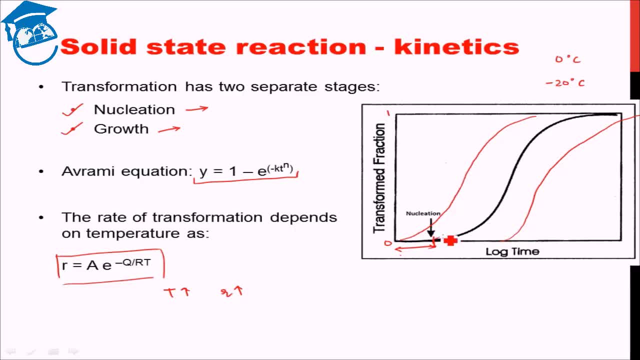 Time of nucleation, then the sigmoidal curve would have been something like this, Something like this: Faster rate of transformation, Fine. So what we saw in this slide, to sum up, is transformation takes place in two stages: nucleation and growth. Nucleation rate depends on the driving force, and that growth stage depends on how fast the diffusion is going to be. 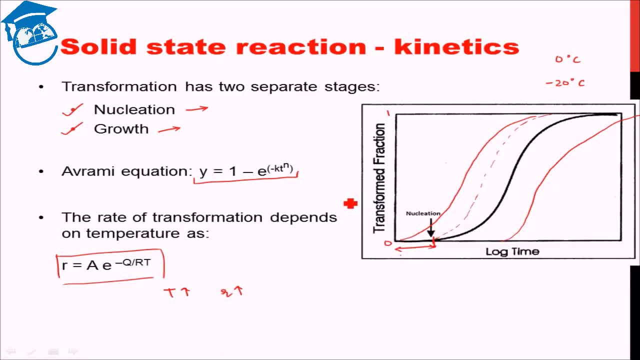 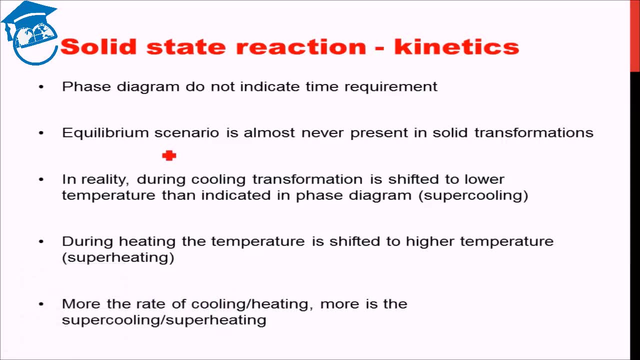 Take place there by on temperature. Now further up, phase diagram, as I said, do not indicate any time requirement because that is by definition considered to be always in equilibrium. It's considered that any diffusion which is required happens instantaneously. But 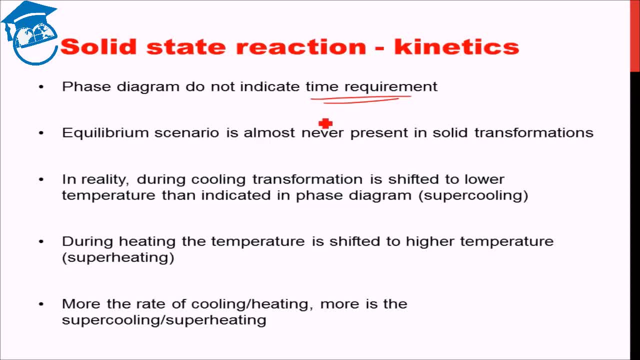 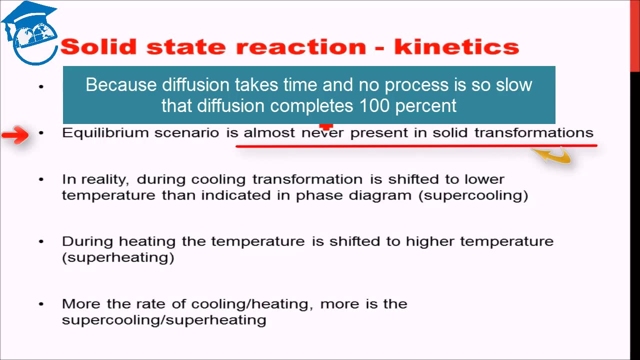 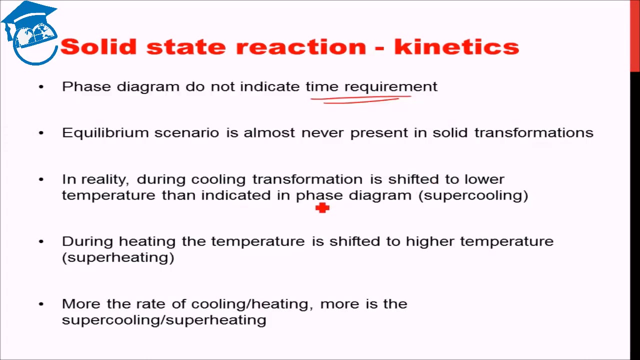 In reality, equilibrium scenario almost never exists during solid transformation, The reason again being that diffusion takes time and any process is never that slow that diffusion can complete 200%. In reality, during cooling, Transformation is shifted to lower temperature than indicated in the phase diagram. 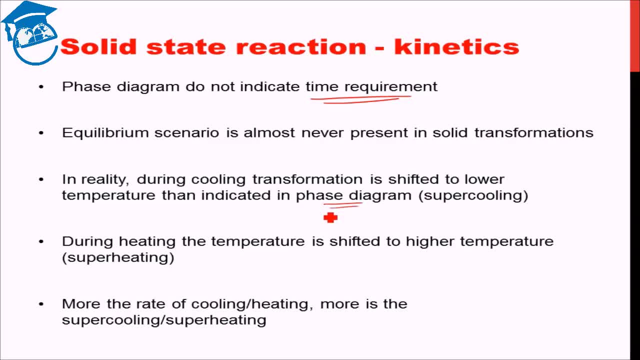 Okay. So now think about this: You Are cooling a thing. Then, if the phase transformation was supposed to occur at 700 degrees Celsius And you are continuously cooling, What will happen is that, because diffusion will require certain time, the transformation will not be able to finish at 700 degrees Celsius. 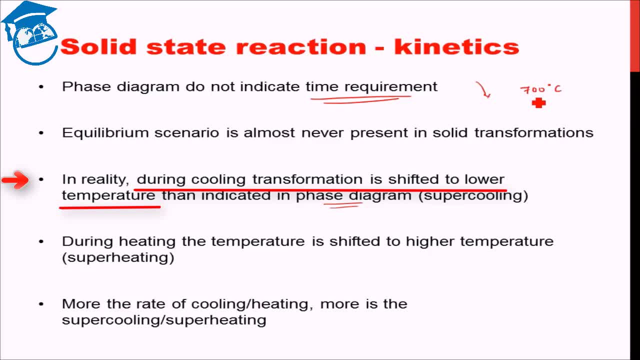 Or maybe even nucleation doesn't start at 700 degrees Celsius. It requires further decrease in temperature. Therefore, in reality, during cooling transformation, There is a shift to lower temperature. Lowering the temperature provides driving force for nucleation. Also, lowering the temperature leads to more. 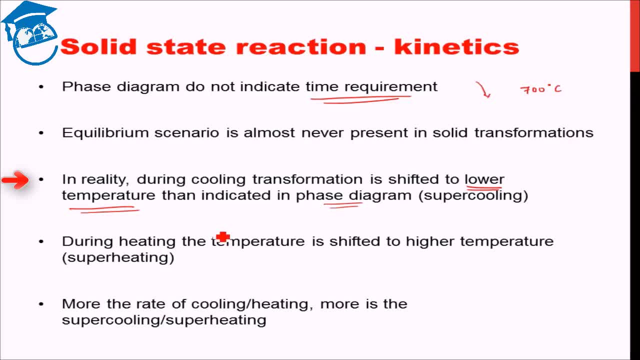 Basically, it leads to a larger driving force, And this phenomena is known as super cooling- Reverse Condition: If you are heating something, Then The temperature for transformation is shifted to higher temperature, And now the term which is used is known as super heating. 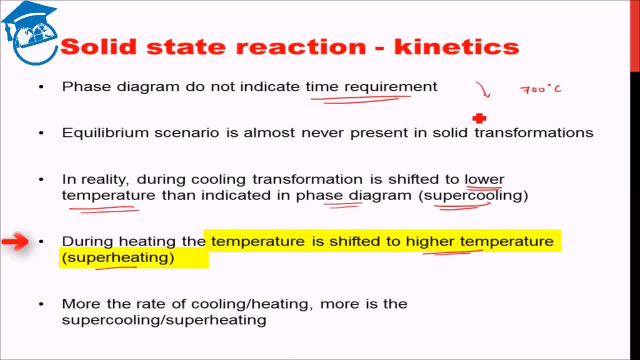 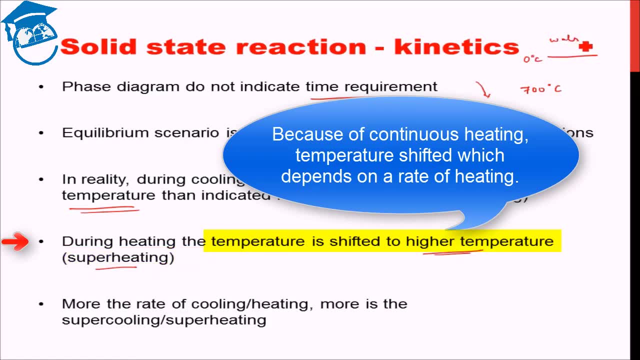 So basically, if let's say We have zero degrees Celsius Water and Ice, Ideally Water should completely freeze At zero degrees Celsius And form ice. But if you continuously cool water, What will happen is that the transformation does not complete at zero degrees Celsius. 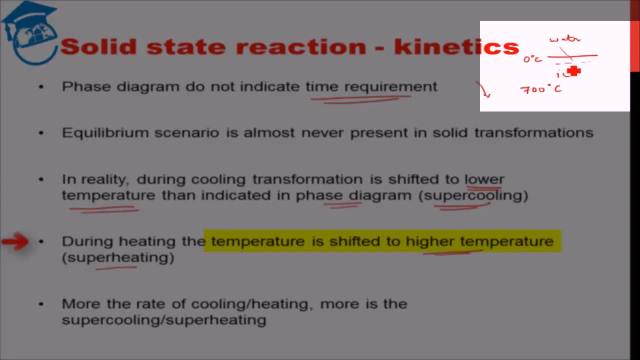 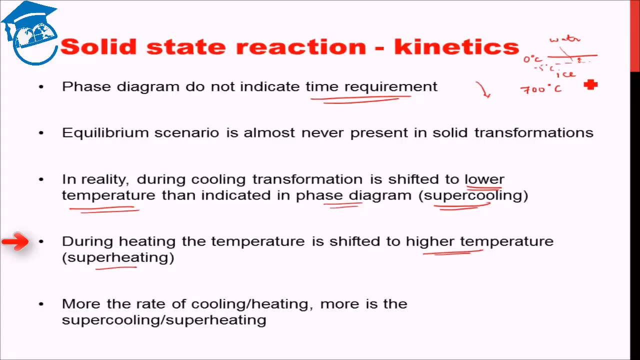 It might complete at, let's say, minus five degrees Celsius due to continuous cooling. This is the super cooling that is taking place Now. you have ice, You are heating it up. It will not melt completely at zero degrees Celsius Because it is continuously heating. 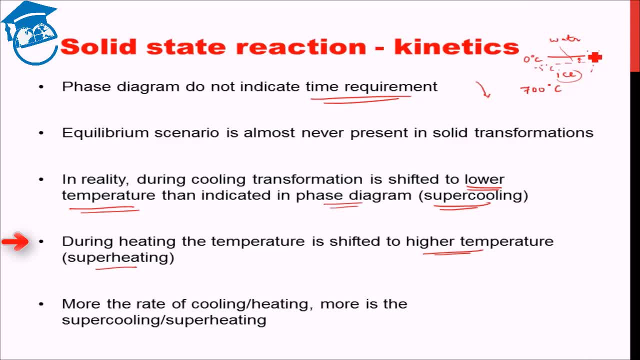 The complete melting might finish at maybe four degrees Celsius, Depends on what is the rate of heating, And this is the super heating that you have done. Okay, And this is exactly the point I was trying to make, That the rate of cooling or heating. 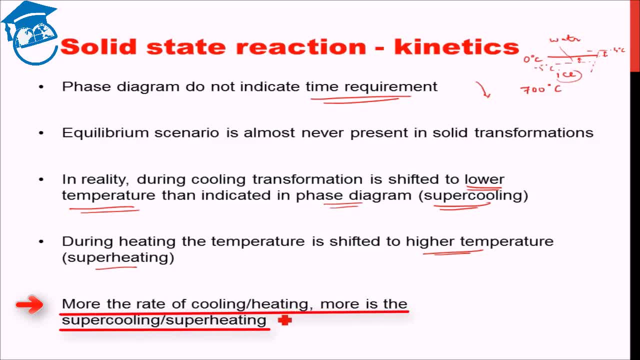 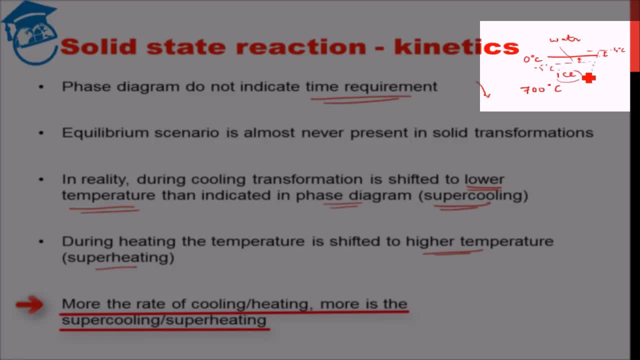 If it is more, Then the degree of super cooling or super heating will be more, Which means That if the water is cooled very rapidly, Then the degree of super cooling may be minus ten degrees Celsius If the ice is heated very rapidly.